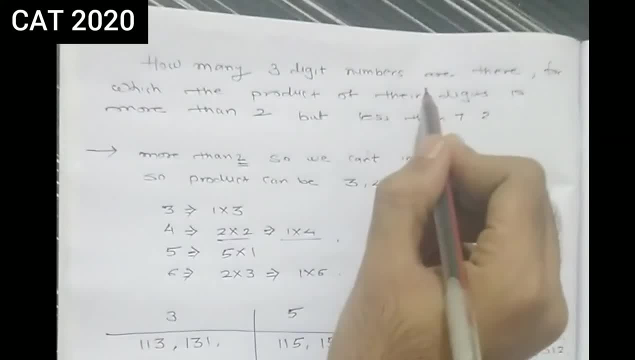 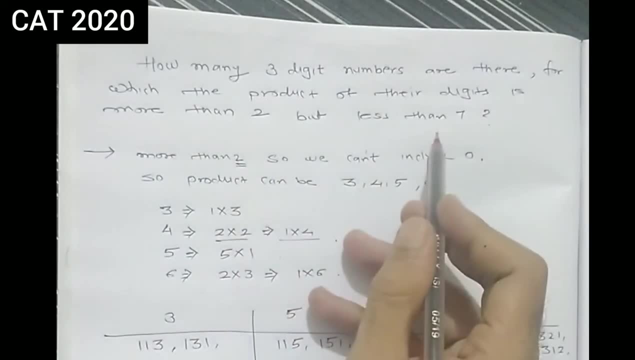 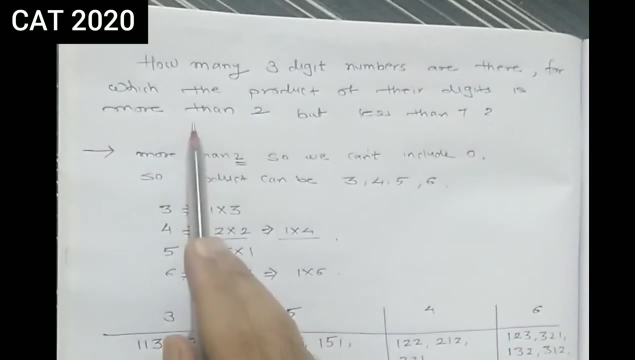 The question is how many 3 digit numbers are there for which the product of their digits is more than 2 but less than 7.. So we want the product of the digits more than 2 but less than 7.. So we cannot include 0 in our number and our product can be 3,, 4,, 5 and 6.. We have factors of 3, 1 into 3.. For 4, we have 2 into 2 and 1 into 4.. For 5, 5 into 1 and for 6,, 2 into 3 and 1 into 6.. 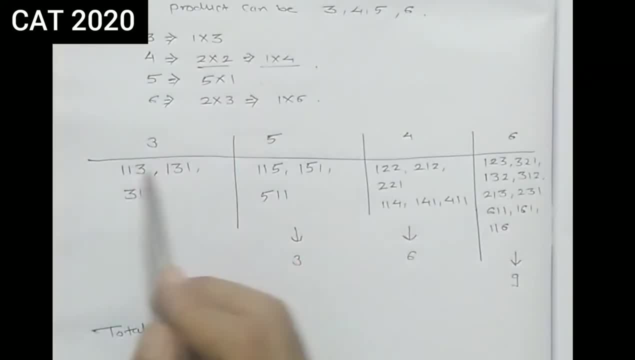 Therefore, we will now form the numbers using these factors. We want a 3 digit number. Therefore, for 3 we can form a number 113, then 131 and 311.. For 5, we can have the factors 5 into 1.. So 115, 151 and 511. 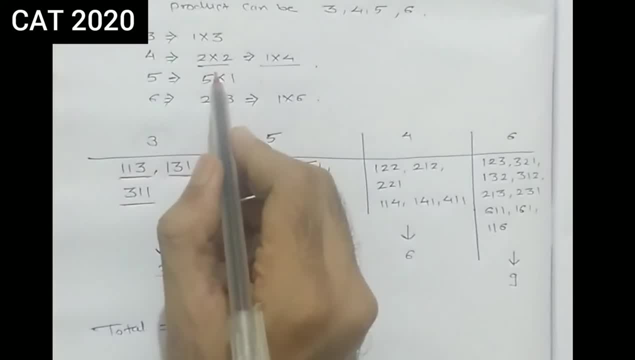 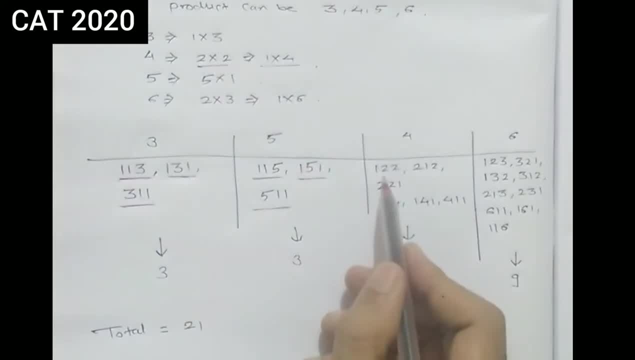 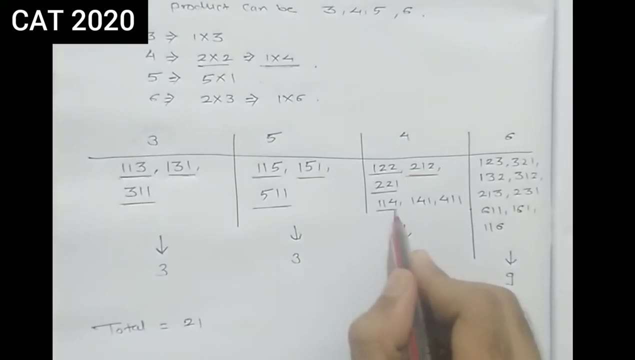 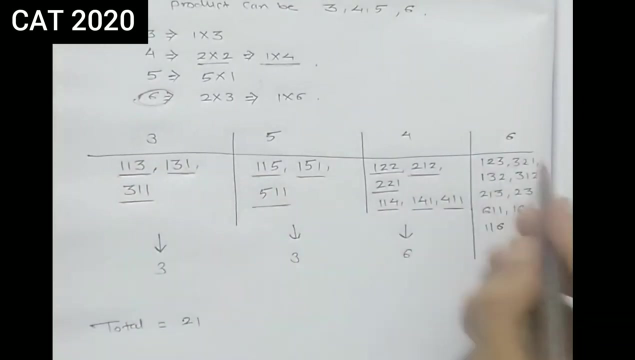 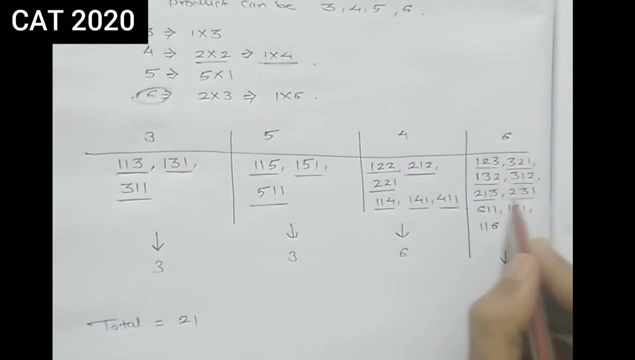 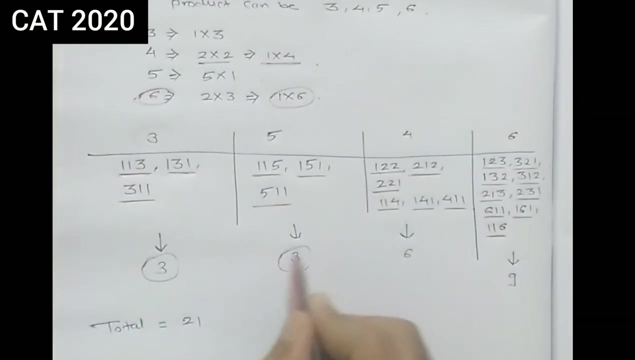 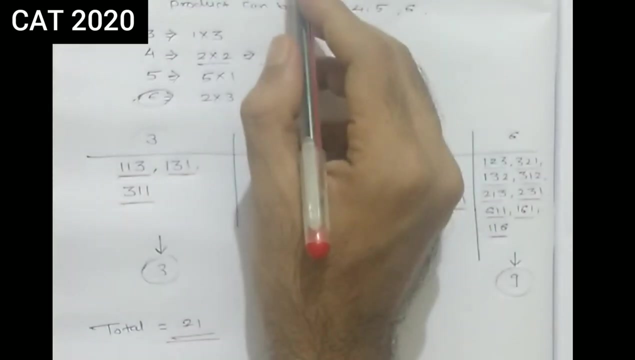 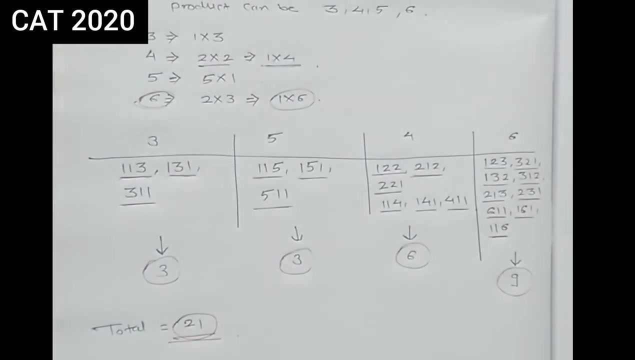